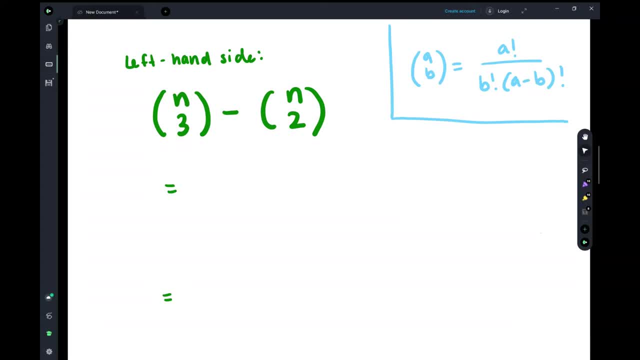 hand corner so we can use as a reference. So, applying this definition to the first term, n 3 we should get. so n replaces the a and 3 replaces the b in this definition. So we should get something like n- factorial over 3 factorial times n minus 3 quantity factorial. So you can see clearly. 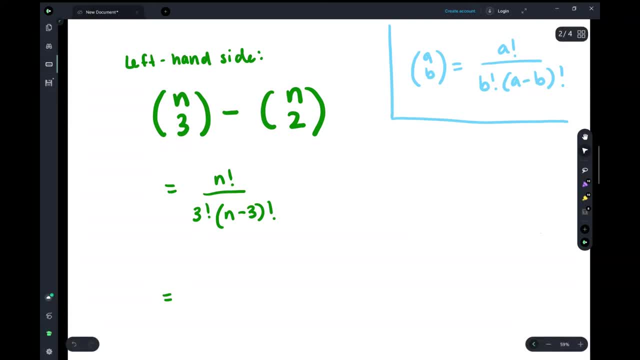 that the n replaces the a and the 3 replaces the b in our definition. Now, doing it to this the next term, we get something very similar: n factorial over 2 factorial times n minus 2 factorial. So now we can further simplify this by playing with these factorials. So when 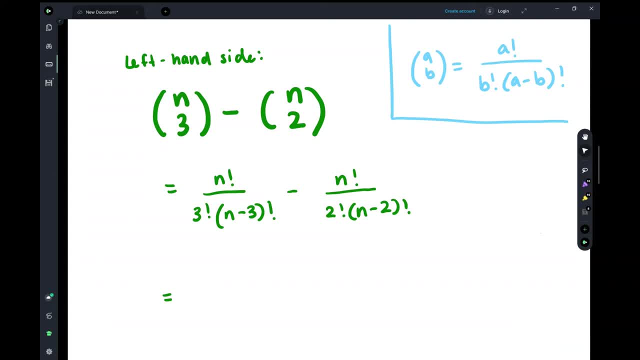 you have factorials in the numerator and the denominator, you should always consider the fact that They might cancel, especially when you have these n terms. So, thinking about what n factorial means, let's just write out that the actual definition of n factorial, which is n factorial, is n times n-1 times n-2 times n-3, dot, dot, dot, dot, dot all. 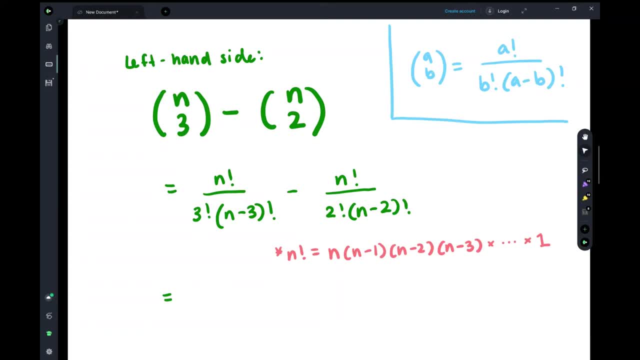 the way to 1.. So essentially n factorial. can you can write it as: n times n minus 1, times n minus 2, times n minus 3 factorial, which will help us simplify the first term, which will give us something like this: so I turned this, I turned this into this because these are: 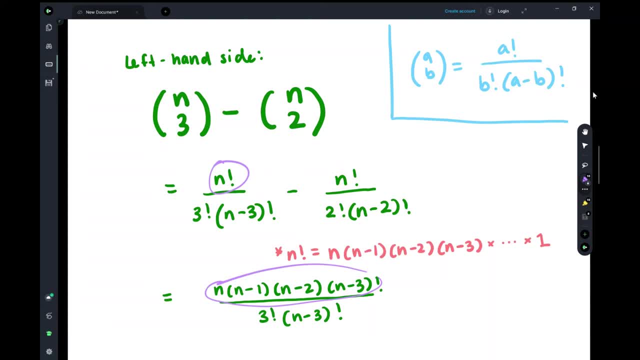 the same and I chose to stop at n minus 3 factorial because we have it in our denominator and in the next step. that'll help us simplify. so we'll just do the next, the same thing for the next term. so doing the same thing for this next term. we can. you guess what? the numerator? 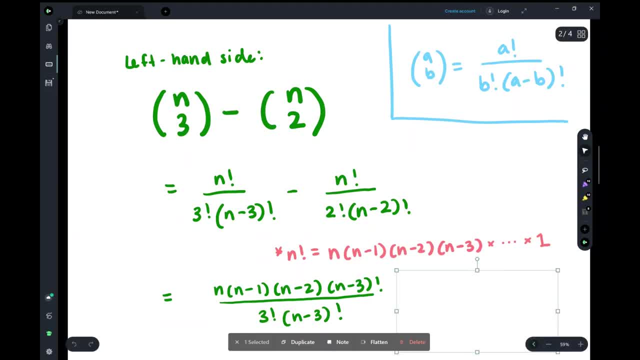 would be, we'll turn into. so basically, it will be the same as this first term, but instead of stopping at n minus 3 factorial, we'll stop one step ahead and we'll stop at n minus 2 factorial. it equals the same thing, but it's just written differently. 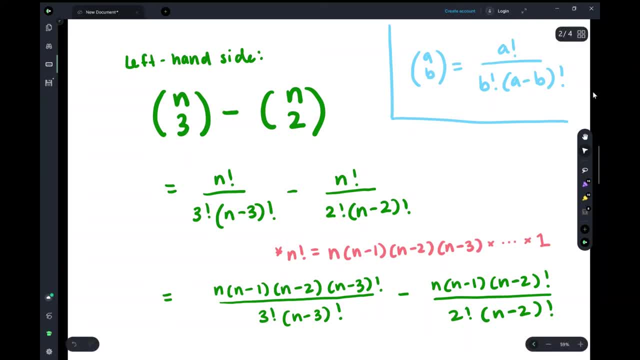 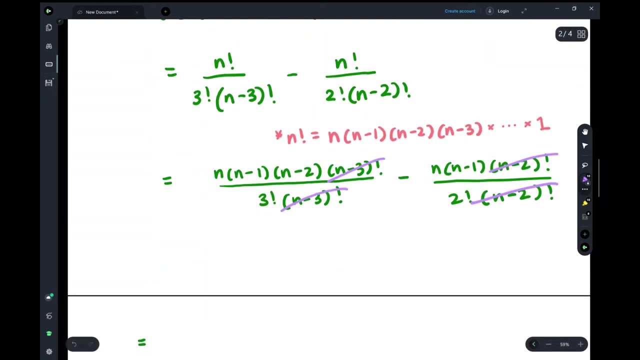 and we're doing n minus 2 because we have n minus 2 in the denominator and now we can cancel, cancel these things like so wrong tool, excuse me. now we can cancel these and we are left with left with a much simpler problem right here. so let's go forward and simplify this even more. so we have we. 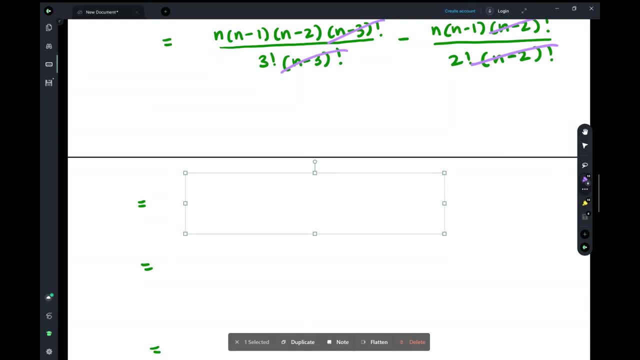 have n times n minus 1 times n minus 2 over 3 factorial and n times n minus 1 over 2 factorial. so that's what we're left with after simplifying and canceling out those, the extra factorial in the denominator. so now simplifying or working these through, the denominators at the bottom turn into: 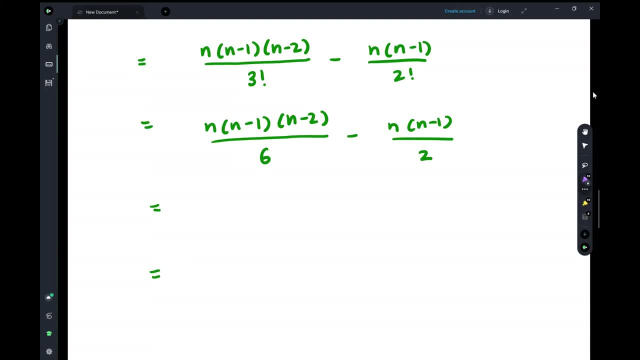 6 and 2, because three factorial is equal to six, two factorial is equal to two. Now we can combine these two terms using a common denominator of six, so that just means we have to multiply this, on this right hand term, by three. 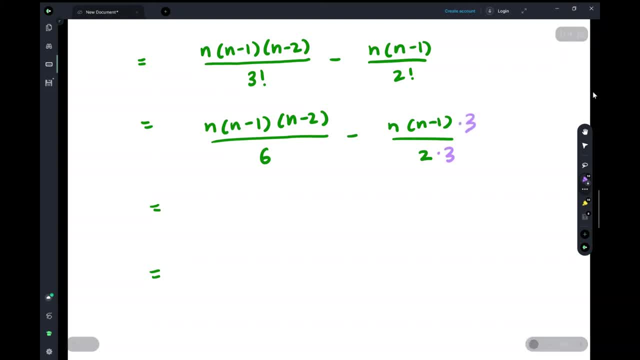 times three, so the denominator will be six and the numerator will just be multiplied by three. so we end up getting something that looks like this: just this numerator minus three, n times n, minus one over six. So now we have one quotient here, and we can just simplify this even further. 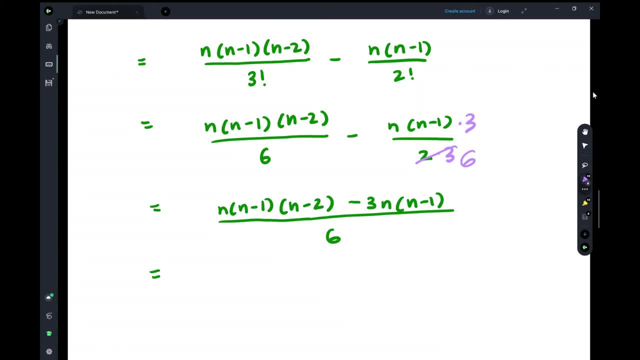 just noticing that We have an n times n minus one here and an n minus n minus one here, n times n minus one. so we can factor that out and factoring that out, we get n times n minus one. times n minus two minus three.